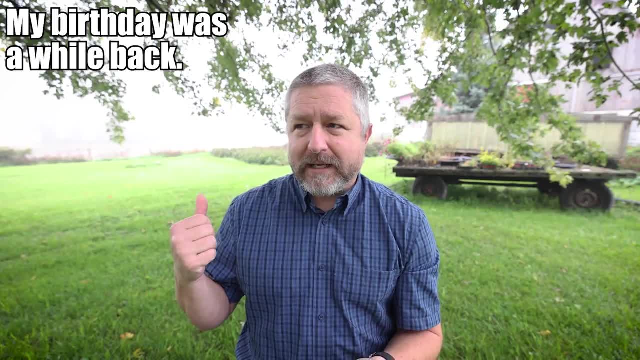 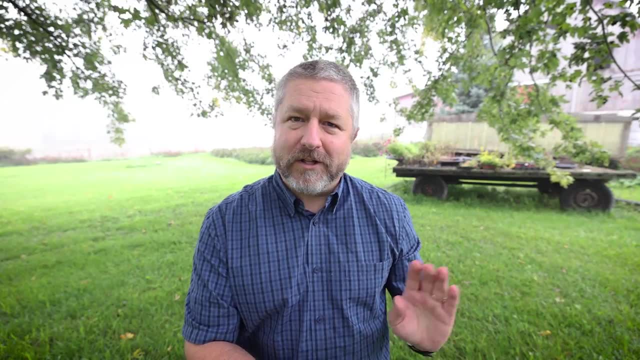 soon, You could say: no, my birthday was a while back. My birthday was a long ways off. It was a while ago. So in English, when you're talking about a future event, you can say a ways off or a long ways off, And when you're talking about a past event, you can say a while ago or 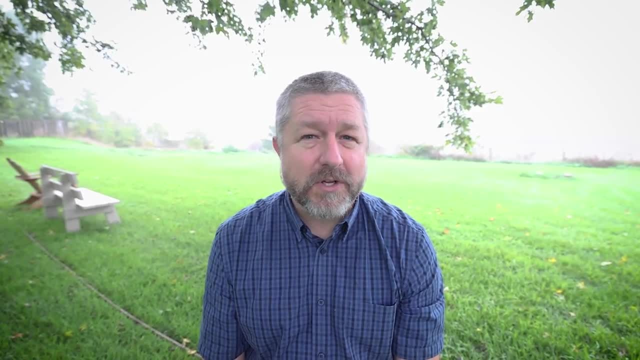 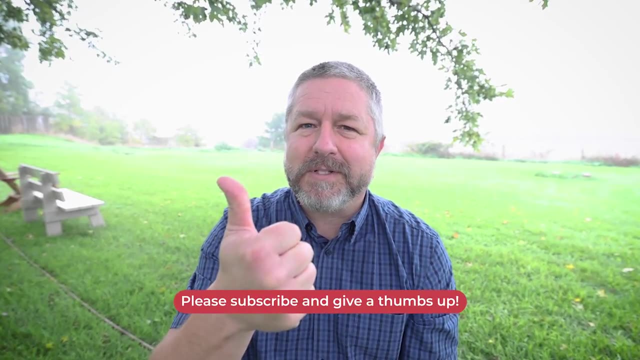 a while back. Well, hey, welcome to this English lesson about time. Before we continue with the lesson, though if this is your first time here, don't forget to click that red subscribe button over there and give me a thumbs up if this video helps you learn just a little bit more English. 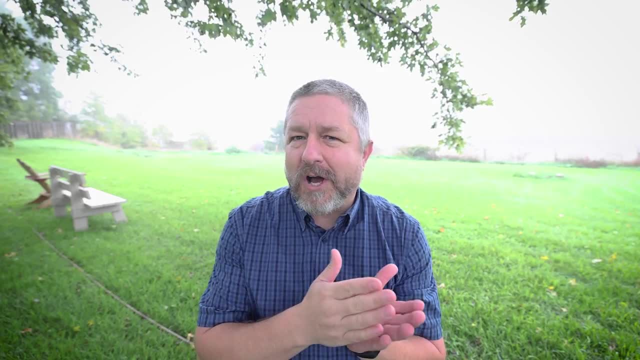 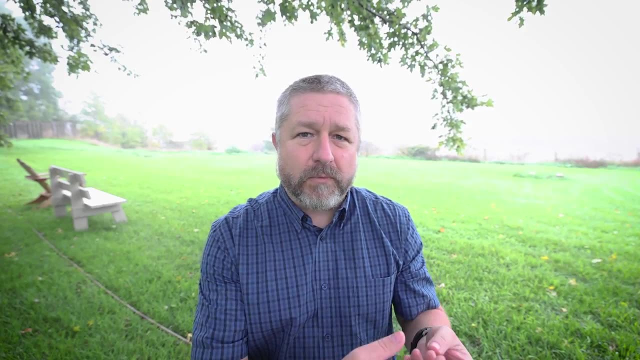 Sometimes when we talk about time, we want to talk about how time goes by really quickly, And there's a few phrases we can use for this in English. Sometimes for me, a certain month will go by really quickly And I would use the phrase that went by fast, And I can be specific. I could. 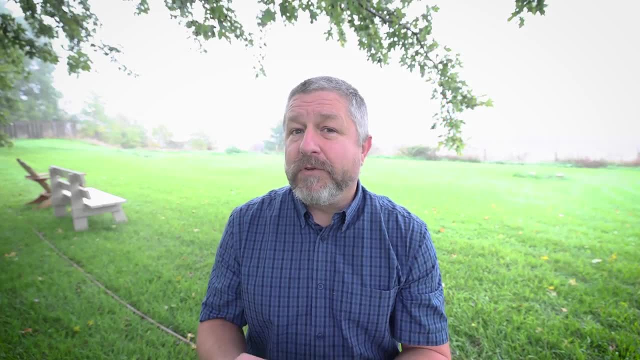 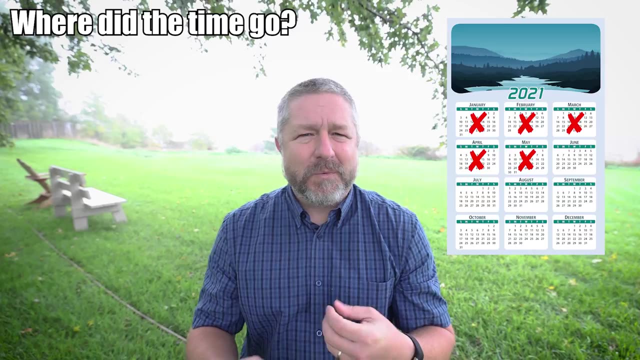 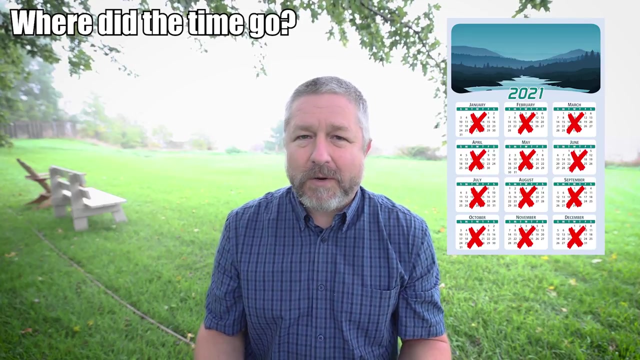 say: wow, that month went by fast And we have a few more phrases as well. Sometimes we ask this question. We'll say: where did the time go? When you say where did the time go in English, you're expressing that something in the past just happened really, really quickly. I could say: 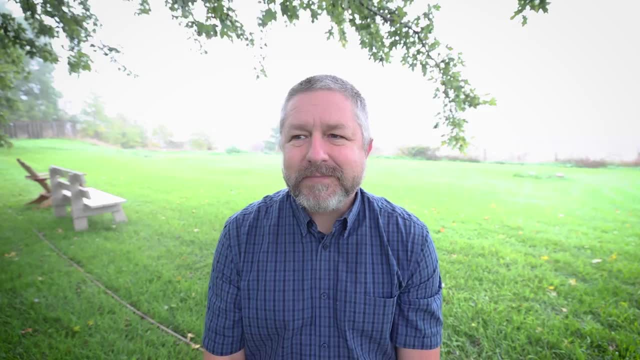 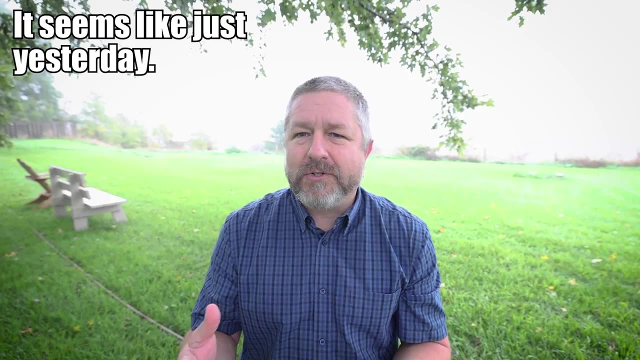 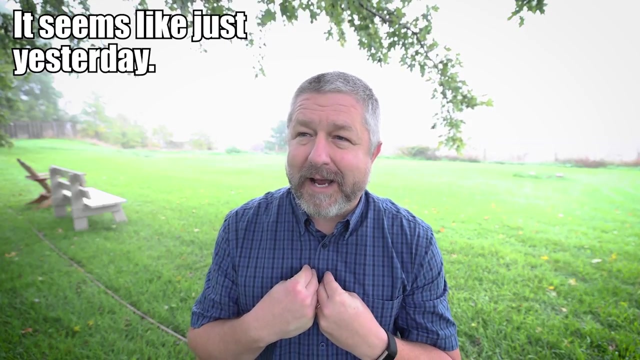 wow, it's already October. Where did the time go? Sometimes we use this phrase as well. We'll say: it seems like just yesterday And we use this phrase to introduce, you know, an idea to the conversation. The best one I can think of is this: Because I have children, I could say: 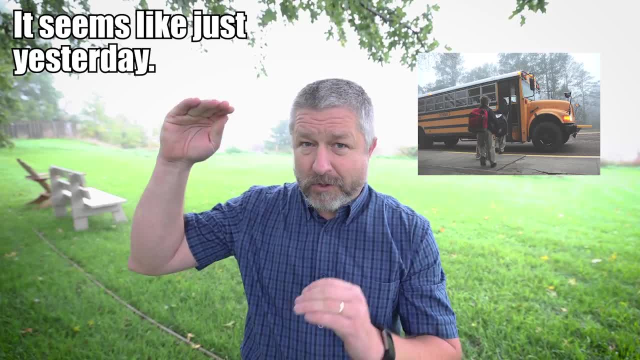 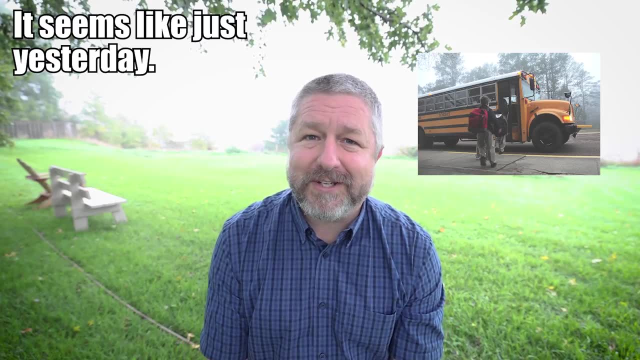 it seems like just yesterday they were really little. They've all grown up quite a bit by now. So sometimes when we talk about how time goes quickly, we'll use the phrase it seems like just yesterday. And there's a phrase that you're probably familiar with: time flies. Sometimes we add time flies when 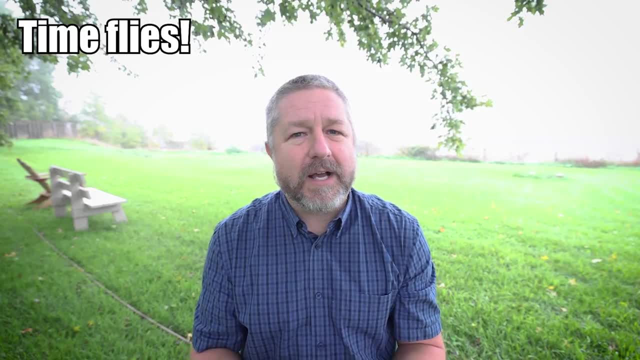 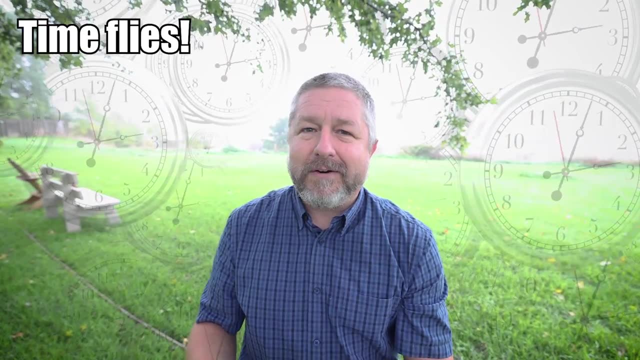 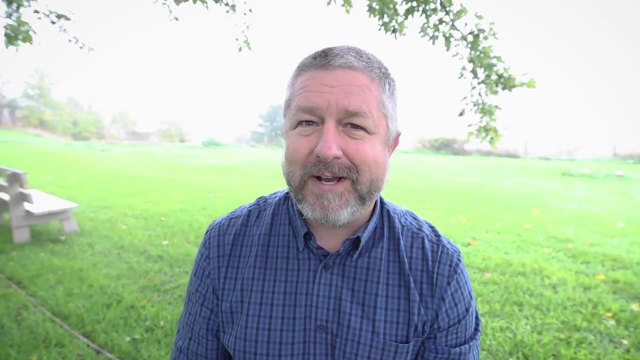 you're having fun, But sometimes we'll just say: oh, time flies, doesn't it? When you talk about a month, that went by quickly, or a year, sometimes a whole year goes by and you're like: wow, it's already 2021.. Wow, time flies. Actually, 2021 is almost over, isn't it? Wow, time flies. 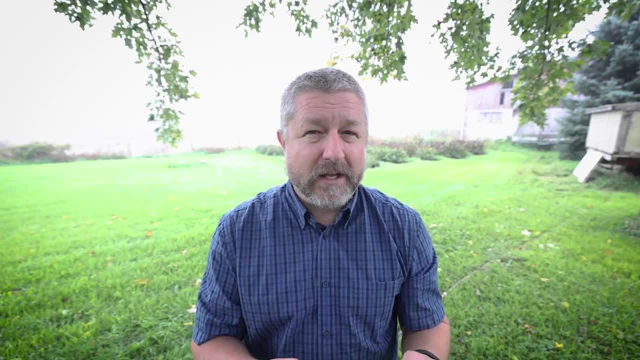 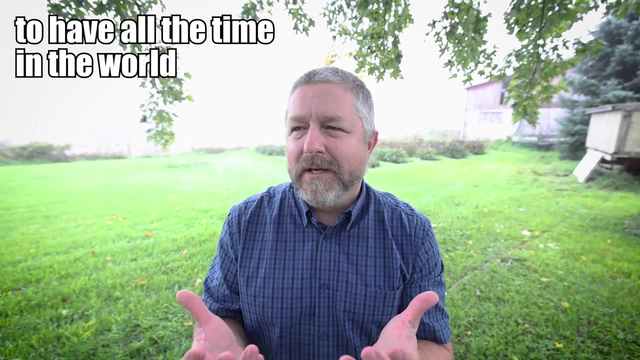 In about 15 years I'll be retired And then I'll have all the time in the world. The English phrase all the time in the world refers to someone who has so much time every day they don't even know how to fill it. They don't know what to do during their day, And this usually 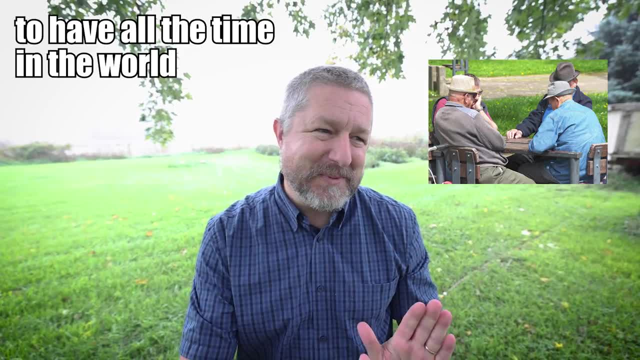 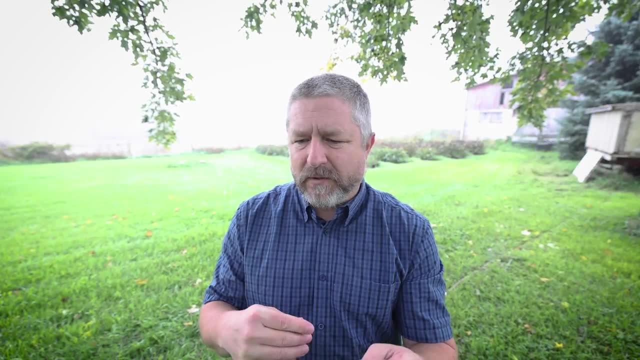 reminds me of retired people. I know retired people are actually busy, but I always think when I'm retired I'll have all the time in the world. Another English phrase we use to talk about having extra time or having time is a little different, and it's the phrase time to kill. 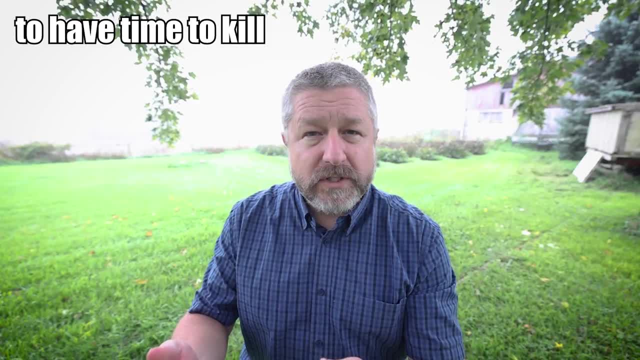 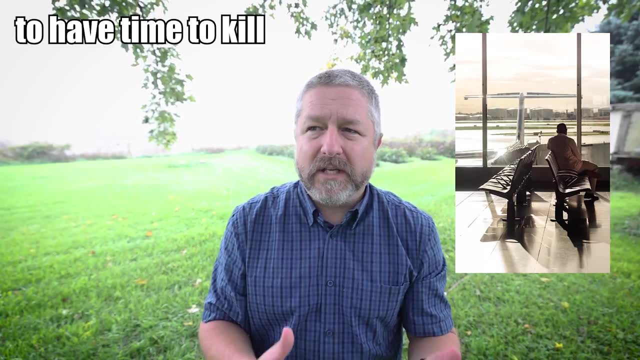 This is a phrase you would use if you were at the airport to pick up your friend and if you found out their flight was delayed by four hours. you would then say: oh, I have time to kill. You have an amount of time where you really can't do. 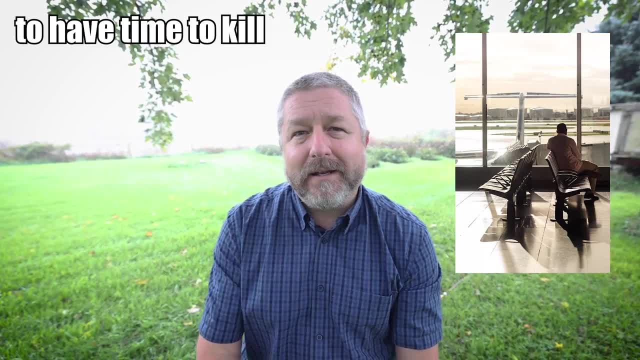 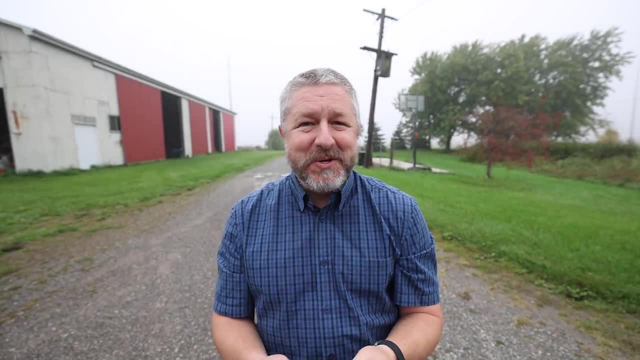 anything else, You need to wait for them. So in that case we would use that English phrase. We would say: you have time to kill. Of course, there's also times when you don't have enough time, where you are in a hurry or you are in a rush, And then we would probably say that you 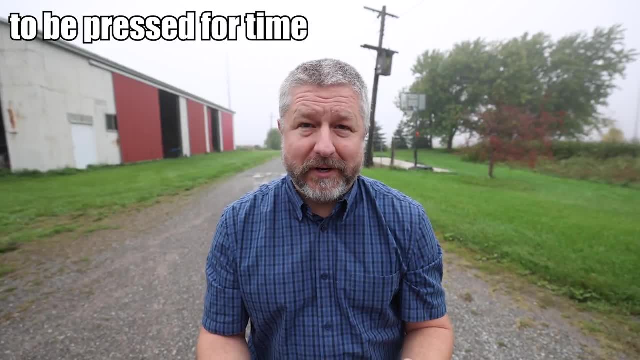 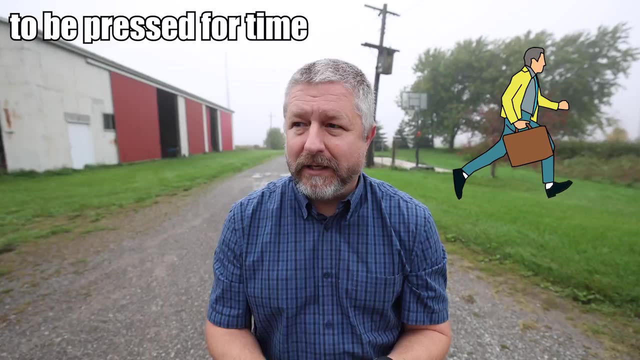 are pressed for time. Sometimes in the morning I'm getting ready for work, I'm running a little bit late and then I'm pressed for time. It simply means that I'm in a rush, I'm in a hurry, I'm going to be late for work if I don't get moving. 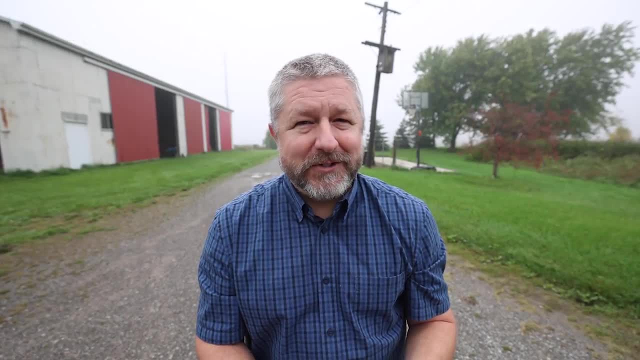 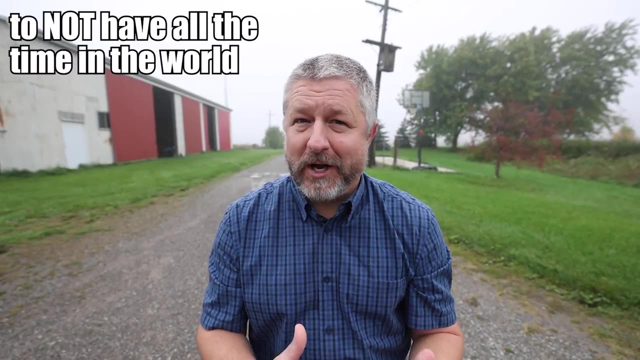 So when you're pressed for time, it means you're probably going to be late for something, And then we also use kind of the negative of a phrase I taught you earlier. We might say that you don't have all the time in the world. This is something that I might say to my children. 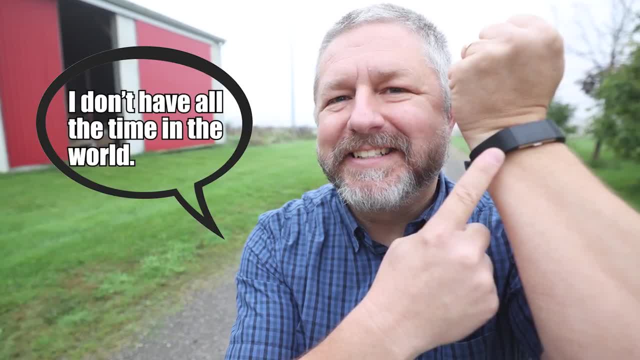 If I'm ready to go and they're not, I might say: let's get going. I don't have all the time in the world, So sometimes you're late, sometimes you're in a hurry and you can use one of those two. 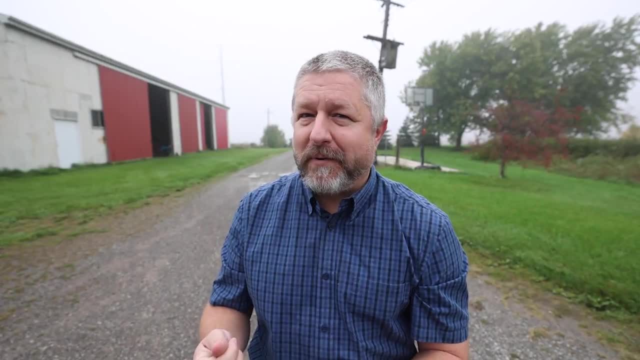 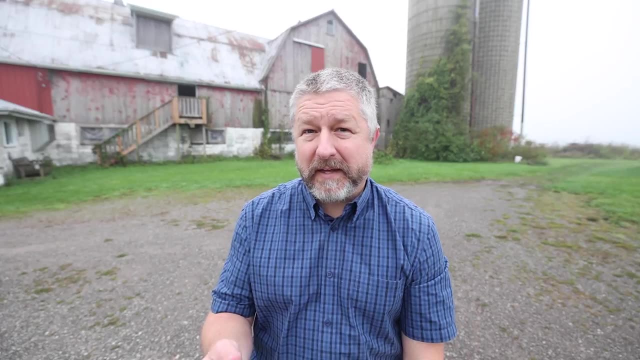 phrases. You could say: I'm pressed for time, or hey, hurry up everybody, I don't have all the time in the world. Sometimes, when you're talking about time, you want to describe something that happened really quickly, like a car accident. In that situation, you would use the English phrase. 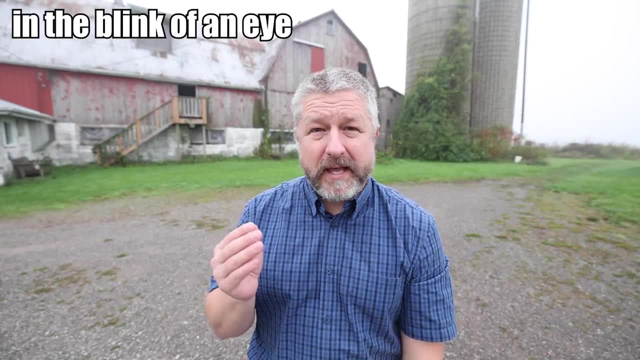 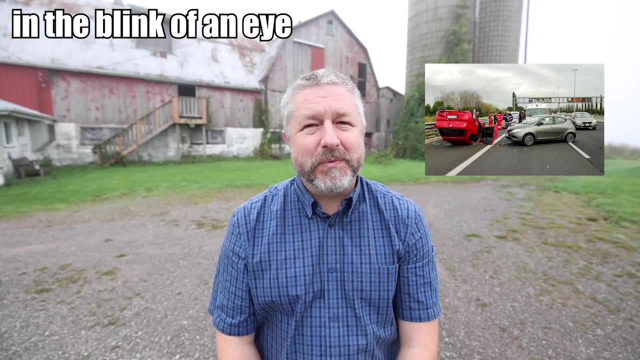 in the blink of an eye. You could say: I was driving along and then in the blink of an eye someone pulled out in front of me and I hit them. That wouldn't be very nice, but that is the English phrase you would use. You would say: it happened in the blink of an eye. Sometimes, when I go to my 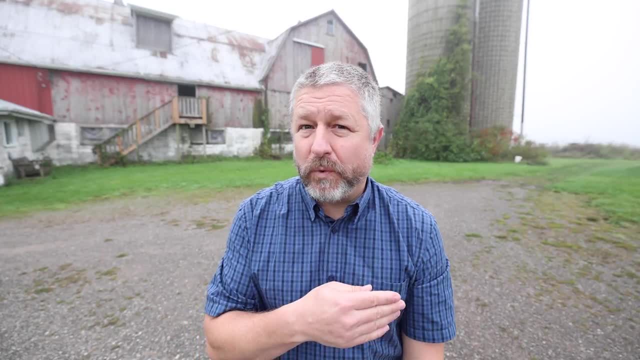 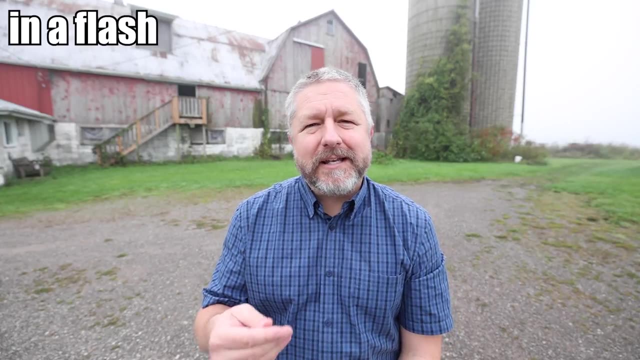 classroom I forget something and I have to go back to my teacher work area to get it. In that situation I would say to students: I'll be back in a flash. The English phrase in a flash indicates that hardly any time will take place for whatever is going to happen. So if it's before class starts, 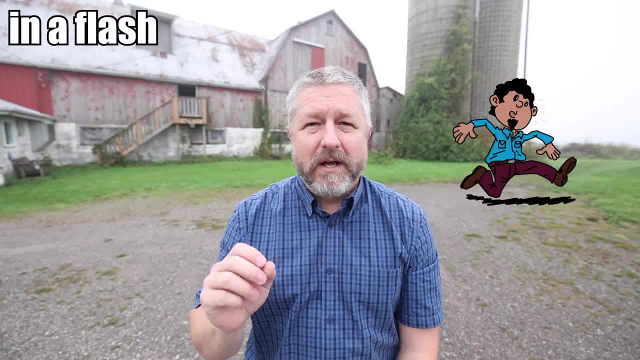 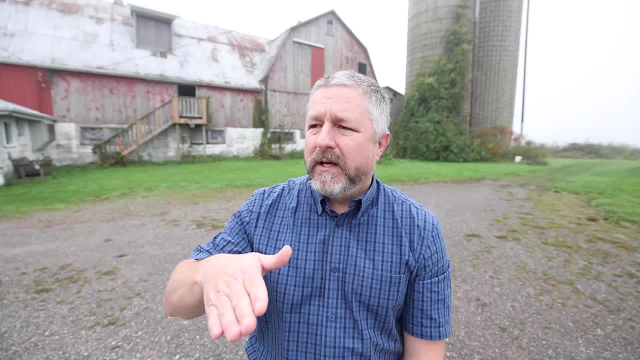 and I'm like: oh, I forgot my laptop. I might say to my students: I'll be back in a flash and then we'll get started on the lesson. Another phrase we use in English to describe when someone does a job quickly is to say that: 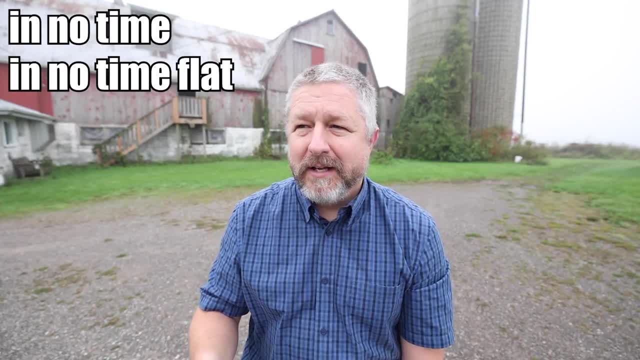 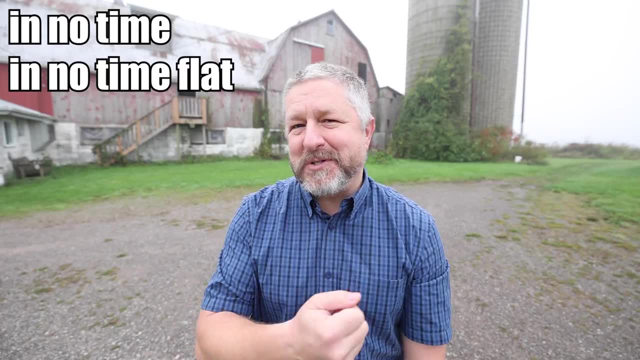 they did it in no time or they did it in no time flat. Sometimes, when I go out to make my English lessons, I'm done in no time. I'm done in no time flat because the words come to me very easily. Surprisingly, with this video, I'm not getting this done in no time flat. It's taking a lot longer. 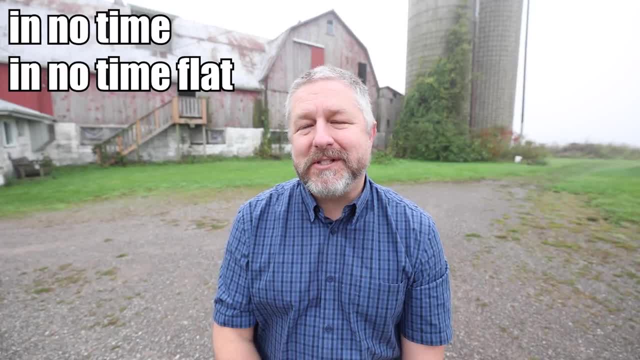 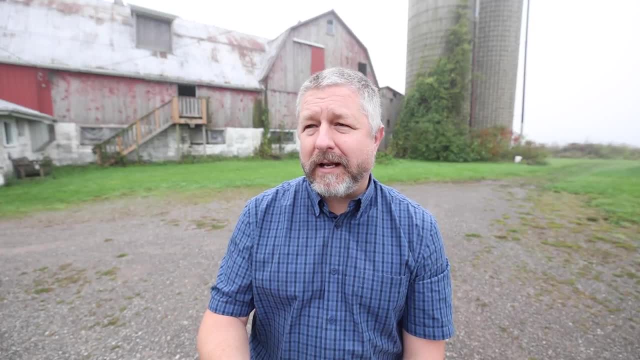 than I expected because I keep mispronouncing words for some reason, But normally when I make these English lessons I'm done in no time flat. So I'm done in no time flat, Meaning that it goes fairly quickly. There's a few English phrases we use to talk about things. 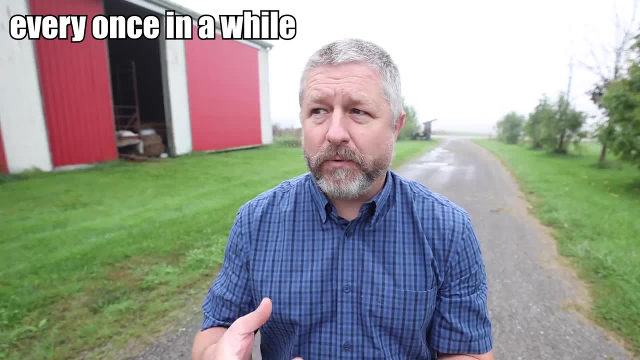 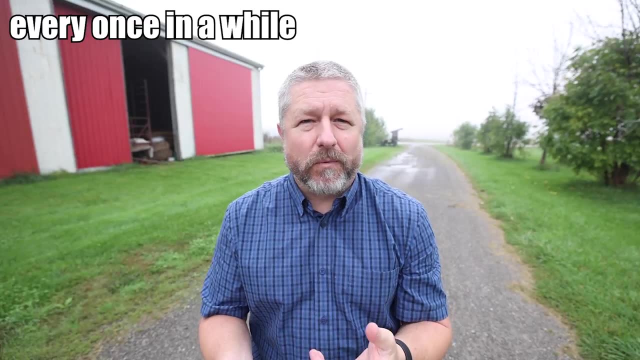 that happen occasionally. We say things like this every once in a while, or from time to time, or once in a blue moon. Let me give you some example sentences. Every once in a while, we take the kids out for ice cream. That means we don't do it every day, We don't do it every week. 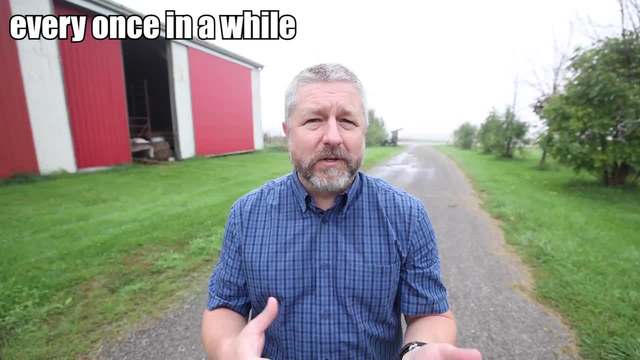 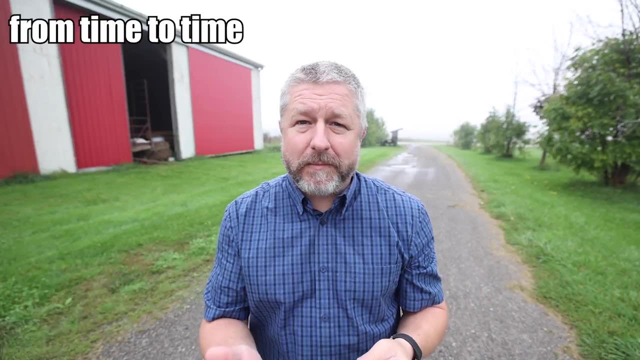 but we do it once a month, maybe every other month, Every once in a while, we take the kids out for ice cream. Another phrase we use is the phrase from time to time, And I could say this from time to time. 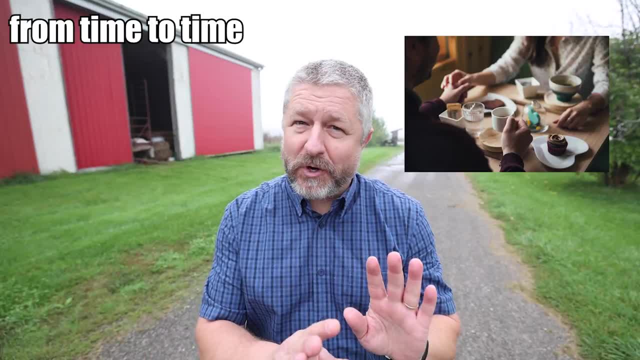 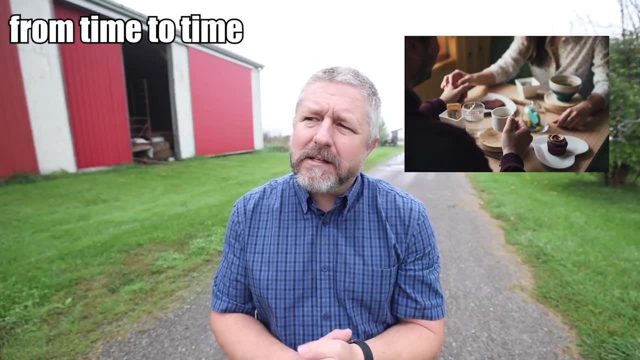 Jen and I go out on a date From time to time. we leave the kids at home and we go out with just the two of us for a meal and maybe to see a movie. So from time to time means, I guess, every other month or so, maybe every three months. There's no specific time attached to these phrases. 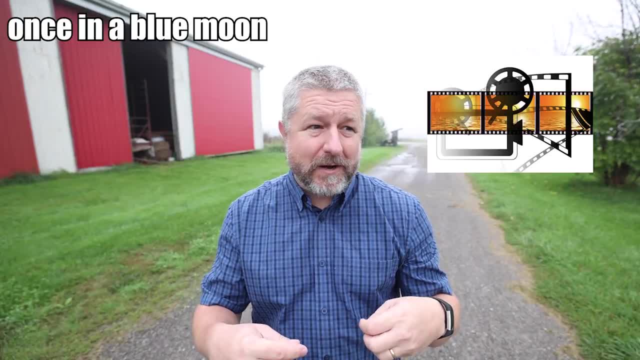 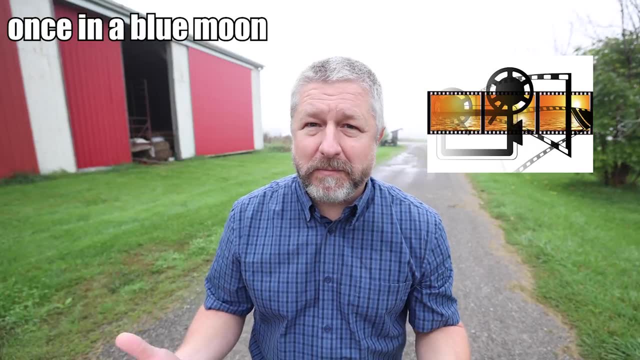 And then the phrase once in a blue moon. When I was younger I went and saw movies with my friends all the time, but now I go once in a blue moon. It means that because I'm older and I'm married and I have kids, I'm really busy. I don't actually